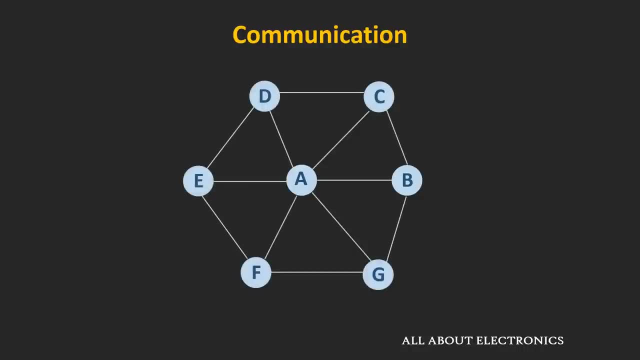 it could be in the network also, And many times this communication could be even the broadcast also, where from one station the information is broadcasted, And one such example is the FM transmission, where a radio station broadcasts the information at a particular frequency and anyone can tune their receiver to the particular frequency. 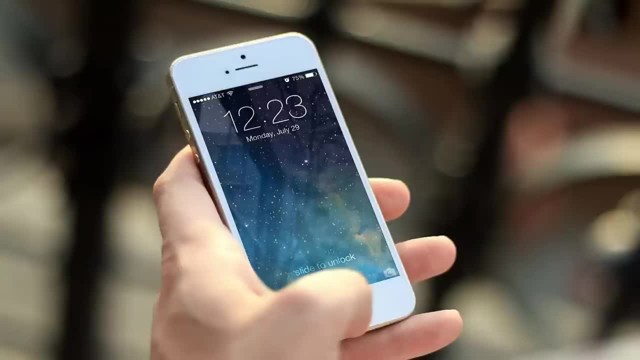 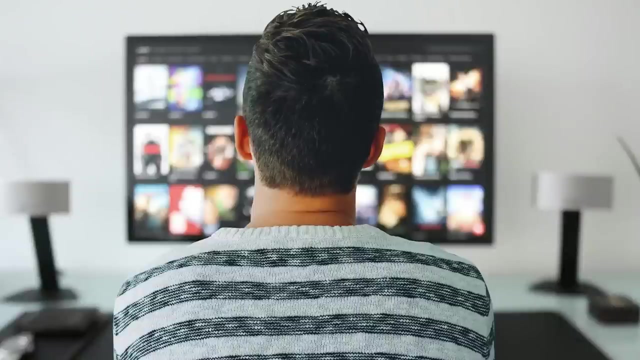 or the channel to receive the information And, in fact, using the gadgets, we are sending and receiving the information every day, like talking on a smartphone Or sending an email to someone, And even watching the television are the examples of the different communication system. 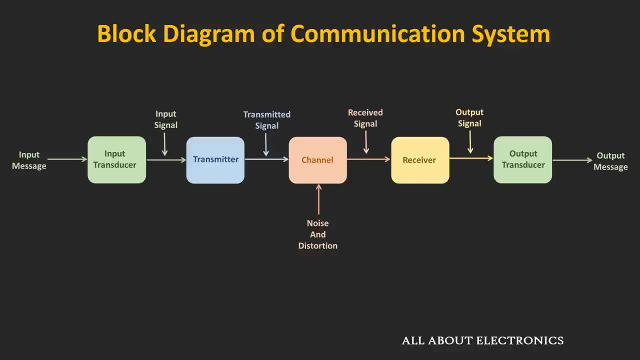 So through a basic block diagram of the communication system, let's understand how the information is exchanged between the two points. So in this block diagram, the first block is the source itself, from where the message signal is generated. So this message could be voice email or the television signal. 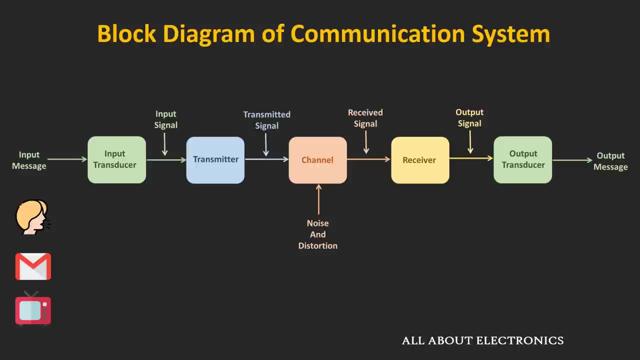 Or it could be even some data signal. So if this message is in non-electric form, then using the transducer it is converted into the electrical signal. So the microphone, CCD camera and the computer keyboard are the examples of the transducer. 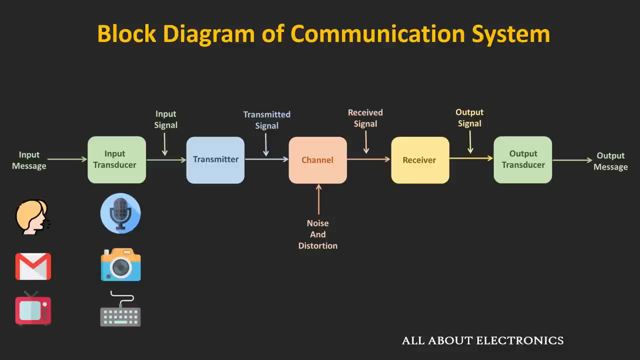 For example, using the microphone, our voice can be converted into the electrical signal, And using the camera, the picture or the motion can be converted into the digital signal. So, after this transfer, the voice will be converted into the electrical signal. 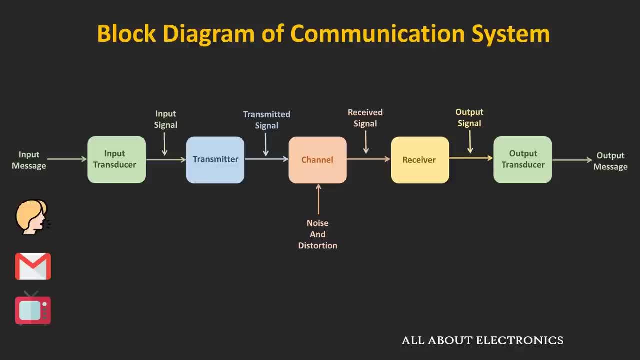 After this transducer, the electrical signal which we have is known as the input signal. Then, after this transducer, the next block is the transmitter. So this transmitter modifies the input signal for the efficient transmission, And this transmitter module also contains several subsystems. 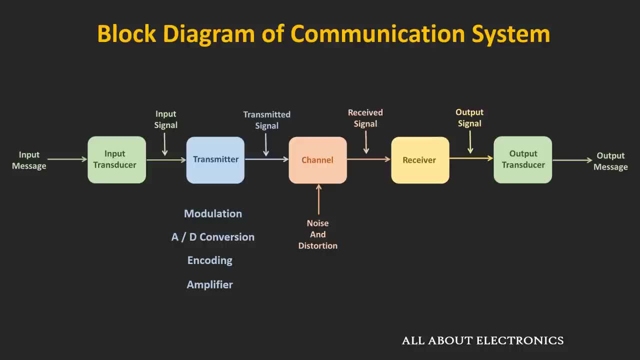 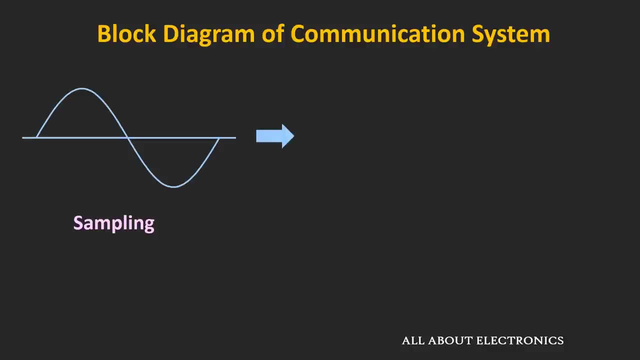 Like the modulator, the analog to digital converter and the encoder, And many times it also contains the amplifier system. For example, if the signal is analog in nature and it needs to be converted into the digital form, then first it is sampled at the regular intervals. 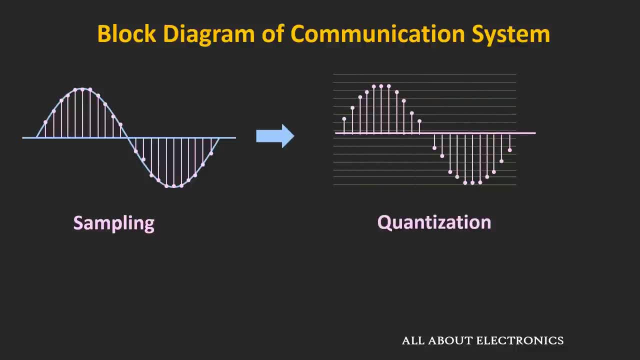 And then it is quantized And after the quantization using the analog to digital converter, it is converted into the digital form And later it can be encoded in a particular format using the encoder And usually, for the efficient transmission, the signal is modulated using the particular 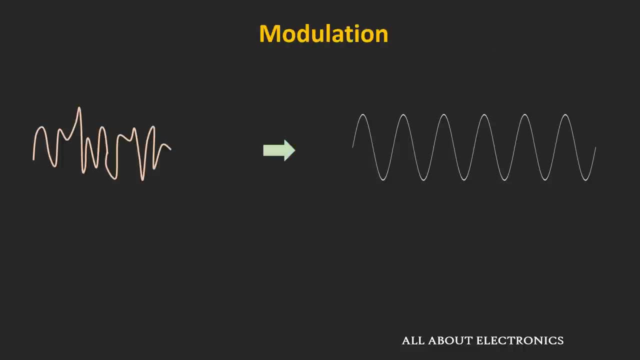 scheme. So this modulation is the process where the property of the periodic signal, like the amplitude, phase or the frequency, is altered according to the input signal. And, of course, in the upcoming videos we will talk in detail about this modulation. So anyway, these are some of the subsystems of this transmitter module. 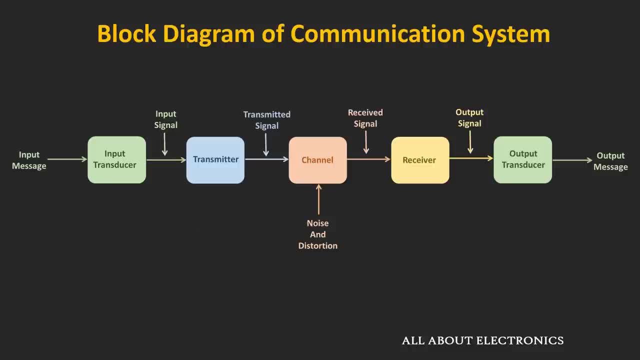 Now, when we talk about the transmitted signal, then we need to know certain characteristics of this transmitted signal, Like whether it is analog or digital signal. So let's talk about the transmitted signal. What is the frequency of the signal? If it contains multiple frequencies, then what is the range of frequencies in the transmitted? 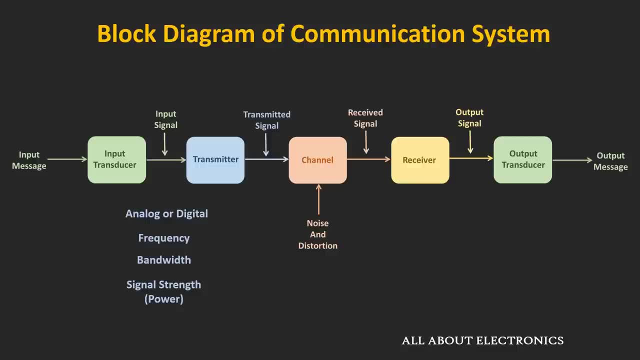 signal. Or, in other way, what is the bandwidth of the transmitted signal And if the signal is transmitted in the digital form, then at which rate the data is transmitted. Or in other words, what is the data rate or the bit rate of the transmitted signal? 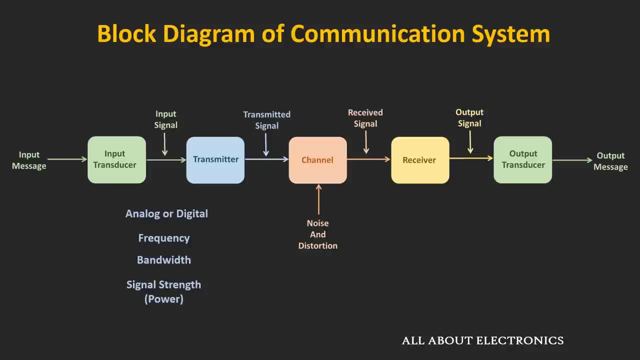 Then another important aspect is the power level of the signal, Because that will decide how long the signal will last, How long the signal can be transmitted over a particular medium faithfully. So these are the some of the aspects which are very important for the transmitted signal. 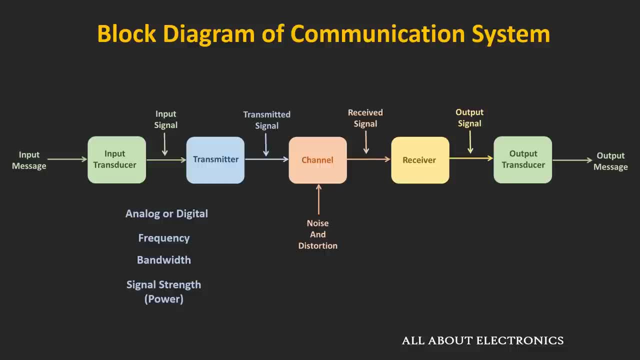 And one needs to see these aspects while designing the communication link. So the signal after this transmitter is known as the transmitted signal And this signal is sent over the particular channel. So a channel is the medium over which the signal is transmitted over the certain distance. 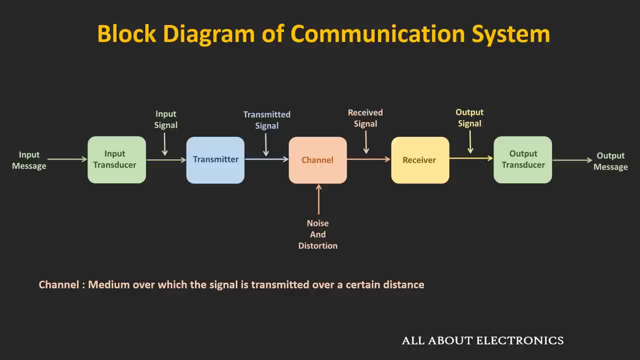 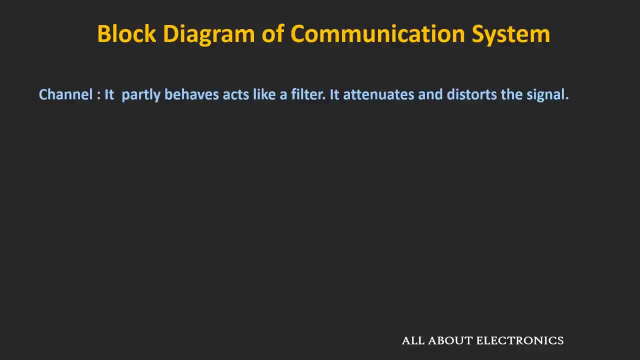 So this channelitus signal over which it has needed signal, is the part of the signal that is transmitted- could be a physical channel like optical fiber or the coaxial cable, or it could be a wireless channel like a radio link. So this channel partly behaves like a filter and attenuates. 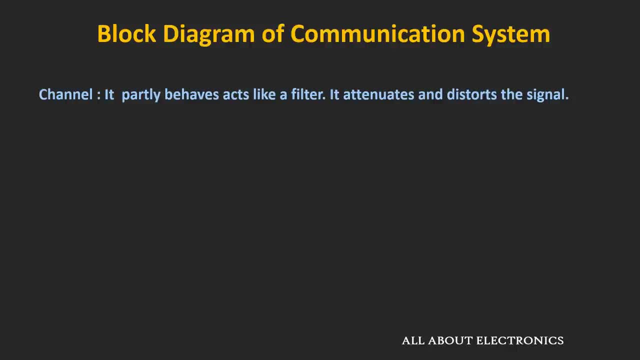 the different frequencies of the transmitted signal differently. So once the transmitted signal passes through the channel and gets received at the receiver, then it gets attenuated as well as distorted. Moreover, the noise also gets superimposed over the transmitted signal. So if this is the transmitted signal at the transmitter end, then at the receiver we may. 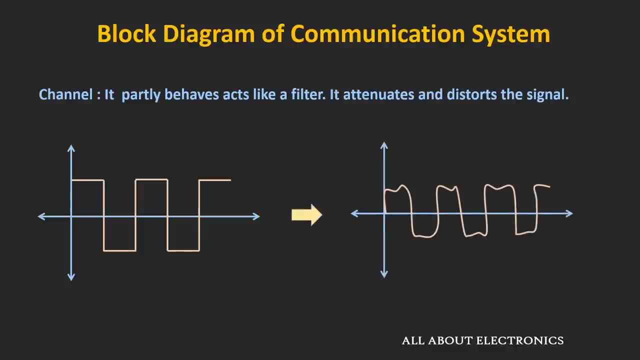 receive the attenuated as well as the distorted signal, And by what amount the signal will get attenuated and distorted will depend on the length of the channel. So if the signal travels longer in a particular medium, then the attenuation and distortion of the signal will be more. But the 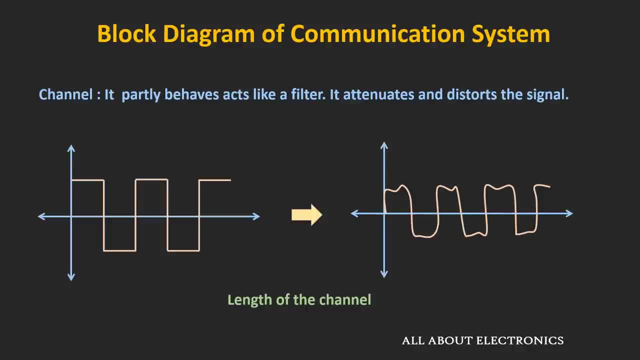 detector or the receiver should be able to recover the message signal from this distorted signal. And whether the detector is able to recover the signal or not, it depends on the signal-to-noise ratio. So it is a very important parameter in the communication system. So this parameter is 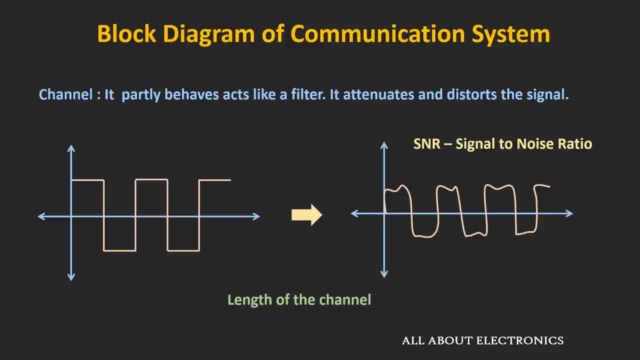 the ratio of the signal power to the noise power. So by increasing the signal power the signal-to-noise ratio can be improved and the signal can be transmitted over a longer distance faithfully. Now, many times the signal needs to be transmitted over a much longer distance. 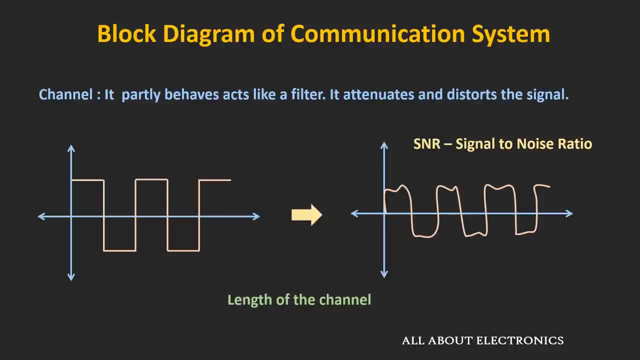 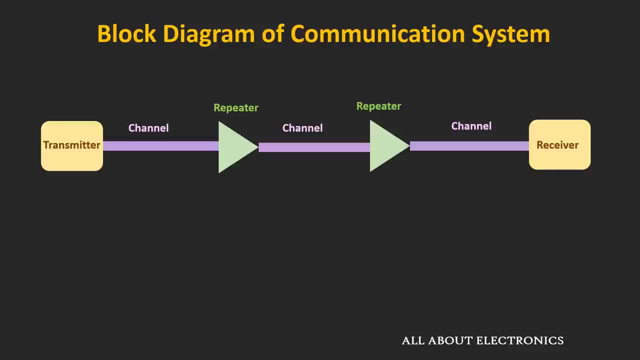 And it is not possible to increase the signal power beyond the certain limit. So in such case regenerative repeaters are used after the certain distance. So these regenerative repeaters detects the distorted and the noisy signal and generates the fresh copy of the transmitted signal And that 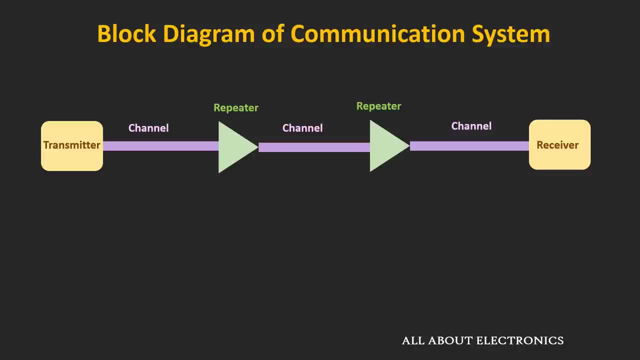 signal is once again transmitted over the particular channel. So this is another way to increase the distance over which the signal can be transmitted, Apart from that, for the digital signals, using the error correction mechanism and by adding the redundancy in the message: signal. 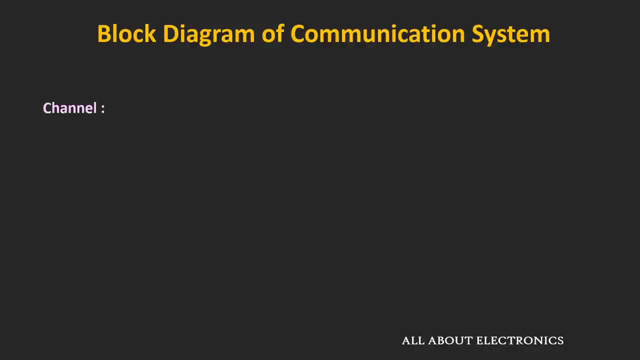 the error in the received signal can be reduced. So for a transmitting medium or a channel perspective. following are the important specifications. The first is: what is the length of the channel, or a distance over which the signal can be transmitted faithfully? Then another: 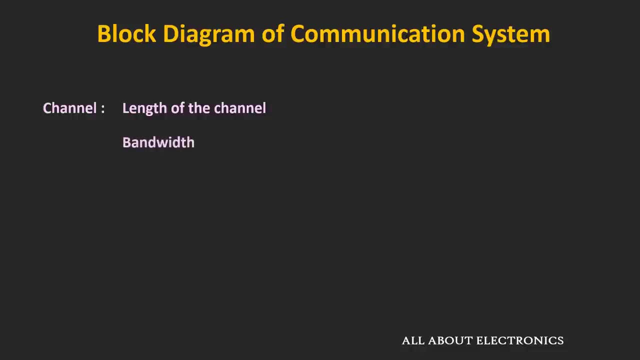 important specification is the bandwidth of the channel, So it is the range of the frequencies which is supported by the channel with reasonable fidelity. For example, if a particular channel can transmit the signal in the range of 0 to 20 kHz, then we can say that the bandwidth of the channel. 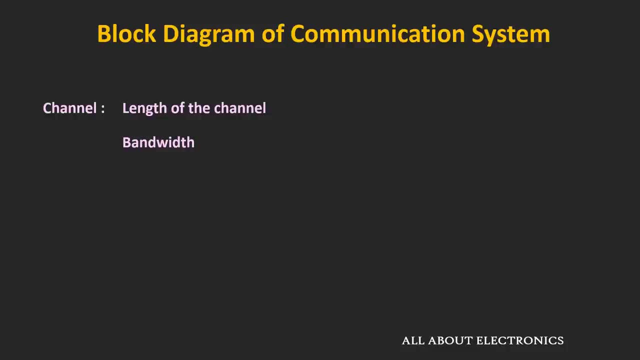 is 20 kHz, And if the signal is transmitted in the digital form, then for the digital signal the another important aspect is the data rate, That is, the maximum supported data rate by the particular channel. So these are some of the important aspects for the channel perspective.